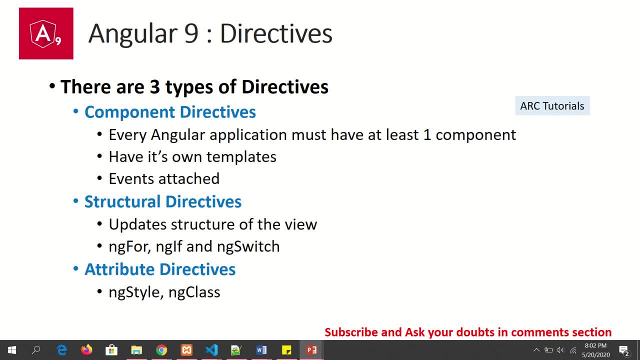 Right. So we can also say that no angular application is complete without a directive. Right Now, component directives have their own templates. Right, We have seen that when we covered that component tutorial in detail, we have seen how to use template URL or template in the component class. 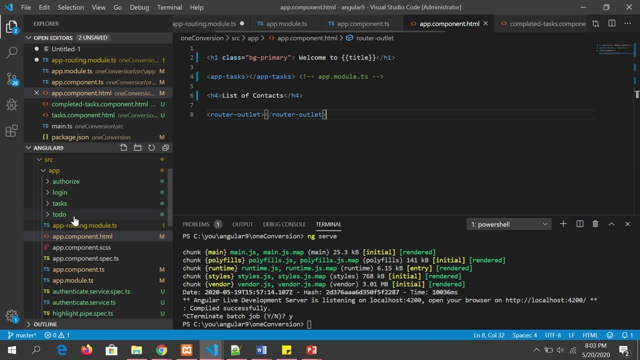 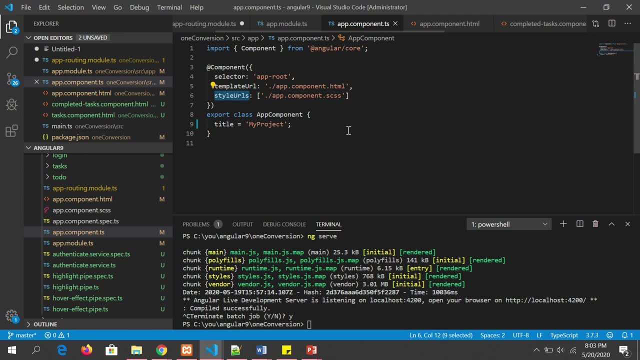 Just to do a quick recap: If you go to your app componentts, you will see the selector, You'll see template URL, You can see style URL. So a component is also a type of directive, Okay, And we can also specify the template. 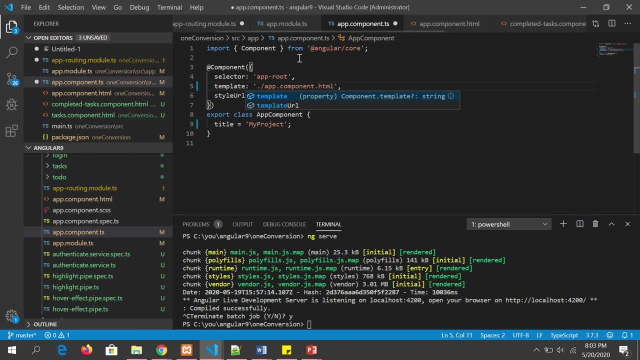 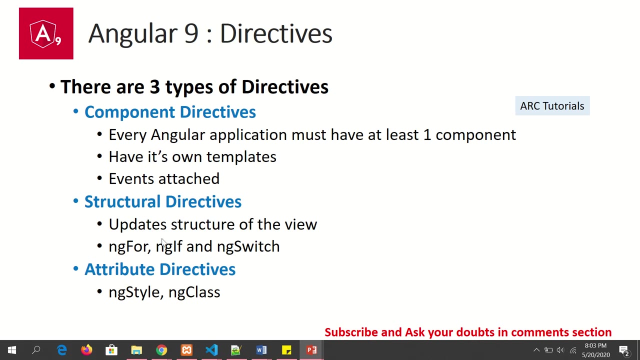 Either You can Just use template or you can use template URL. Whichever you use is fine. The idea is, this directive will have its own template. It will have its own style. That's the important piece. Then we can also attach events to the component directives. 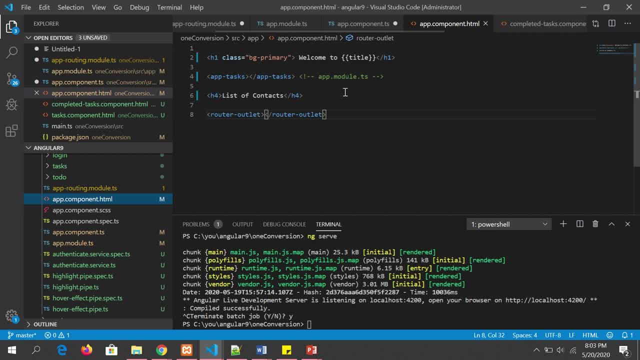 Like, for example, in the HTML we can have. let's say, you want to define a button, Let's do that. So this is how you can define event Right And say: so, this is a button Right. So this is how you can define a simple button that will get displayed and you can implement. 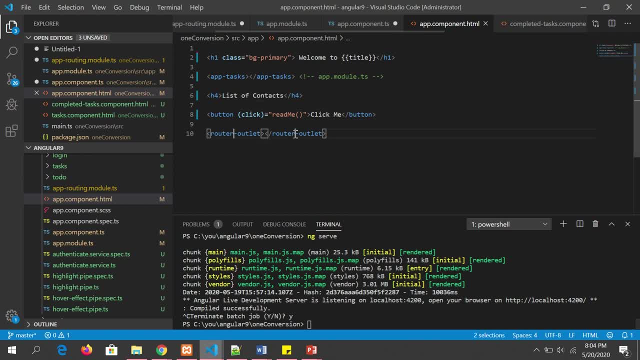 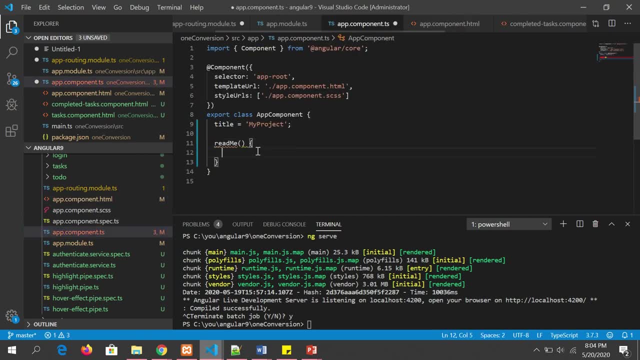 this method in your component. You can just Right, And then you can. just for now, I'm just doing a console log. So you can just Right, And then you can just For now, I'm just doing a console log. 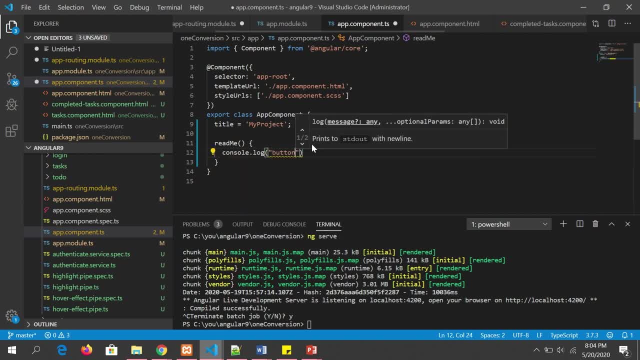 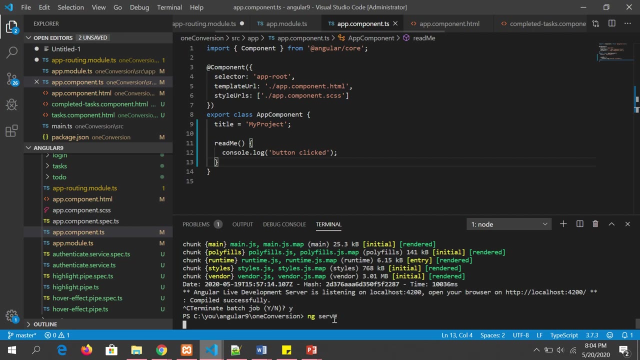 Right, And then you can just Right, Right, Right, Right, Right. It's a good practice to use single quotes. since I've enabled that linting Right, Now let's fire this by starting: ng serve, And you will see that when you click on the button, you will see a console log. 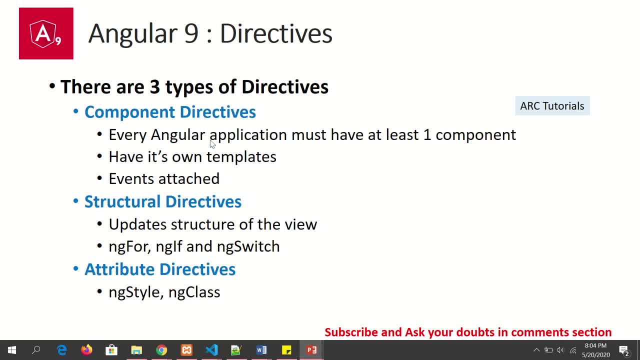 That's straightforward. Now, that is all about component director. A best way. also, if you want to learn, please check out the tutorial on components that we have covered previously. That will give you complete details about the components: What components are, how to generate components, how to use them. 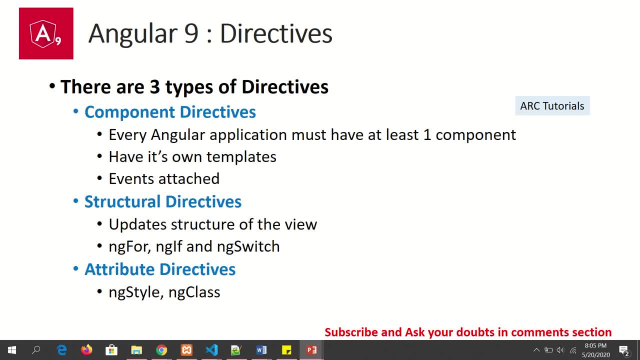 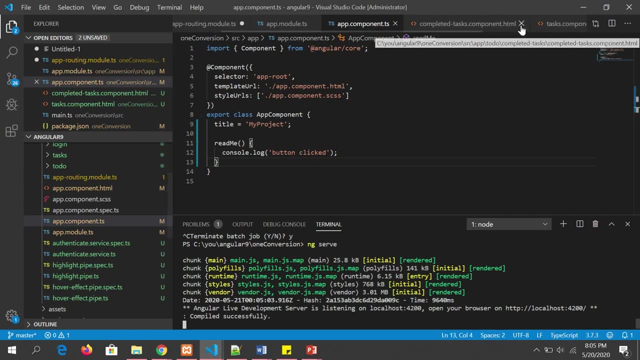 Now the next one is structural directives. This is very, very important because these are used to change the structure of it, Right? So I am going to make some notes for you again. I do that in every tutorial for you, So let me do that here. 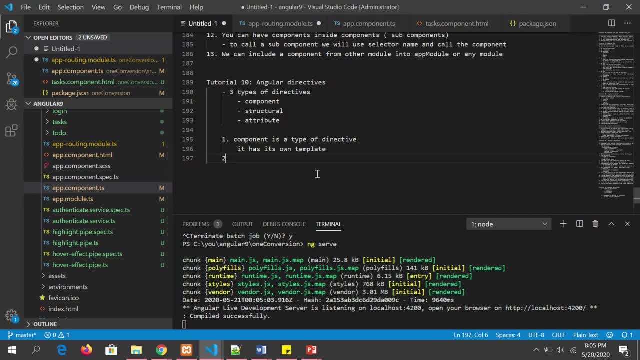 Let me close all of this. So All right. So angular directives. we have three types of directives: components, structural and attribute. component directive is a direct type of directive. It has its own template. No, every angular application must have at least one directive. or we can say component. 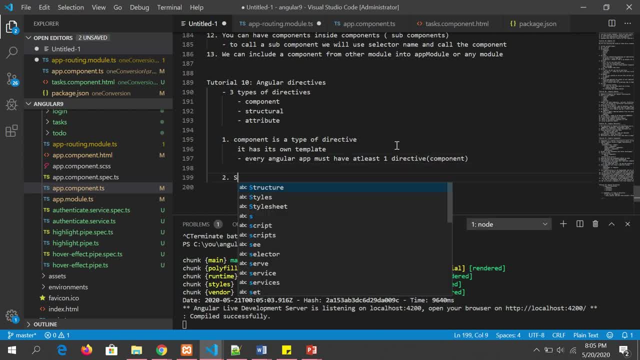 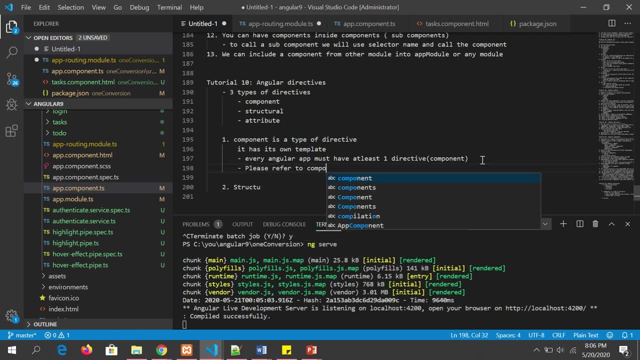 one component right Or one component director. Now let's talk a little bit, And I will also mention, Mention it here, that please refer to components tutorial to learn in depth about components so that, if you see, here we have covered a lot of beautiful um things about angular. 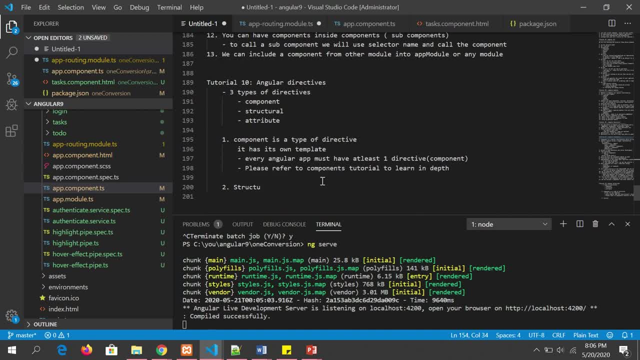 components. We have learned so many things about it, So please make sure you go through that tutorial number. that's number nine, tutorial number nine, and that will help you. All right, So structural directives. So these are very, very important because 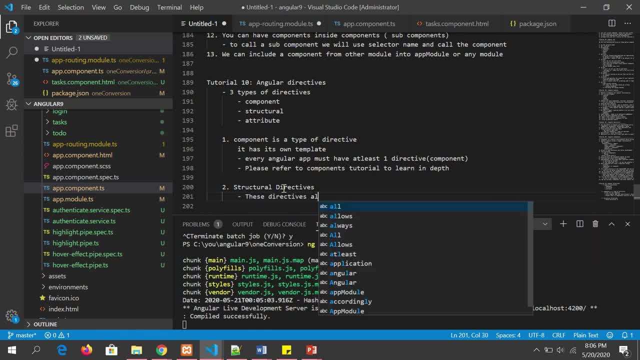 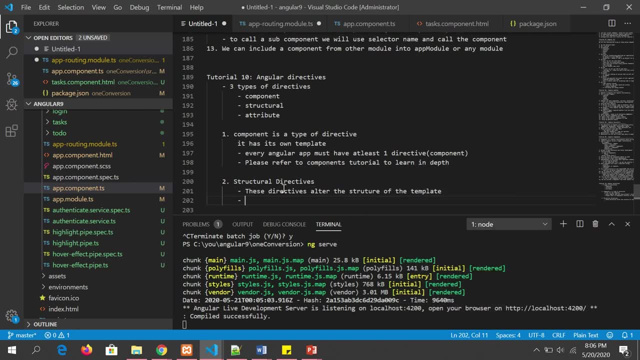 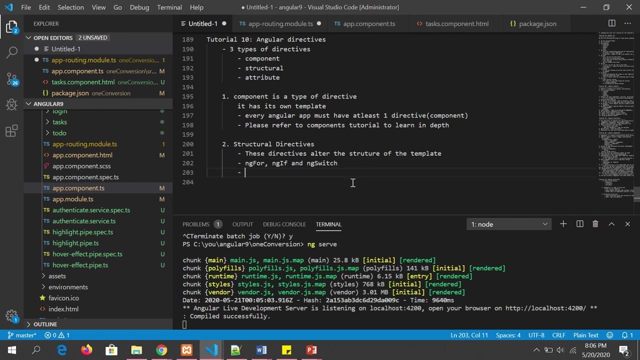 They are. these directives alter the structure, Structure of the template or the view right. Importantly, we'll use NG for NG if and NG switch. These are the three main types of structural directives. Now NG for if you relate to it um you, I'm sure you would have used for loop in any 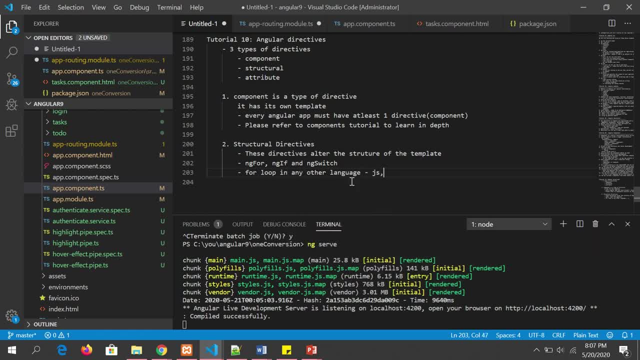 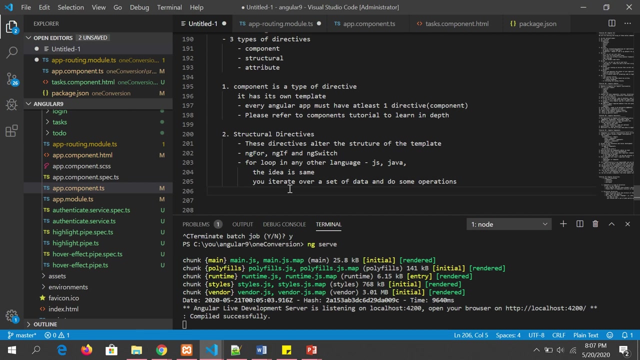 other programming language, Uh, JavaScript, Java or any any language. uh, the idea is same, right, Which is, you iterate, iterate over a set of data and do perform some operations, right? So similarly, we will do the same, um in using NG for right. 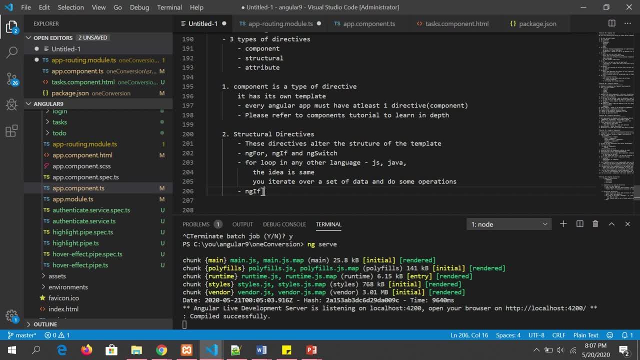 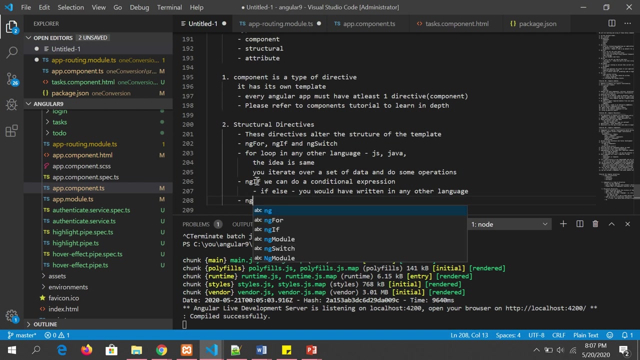 And using NG. if again, um, we can do uh, conditional based check expression checks right. So this is again similar to uh. if else conditions that um you would have written in any other language, any other language. now, NG switch, same same case, like you. 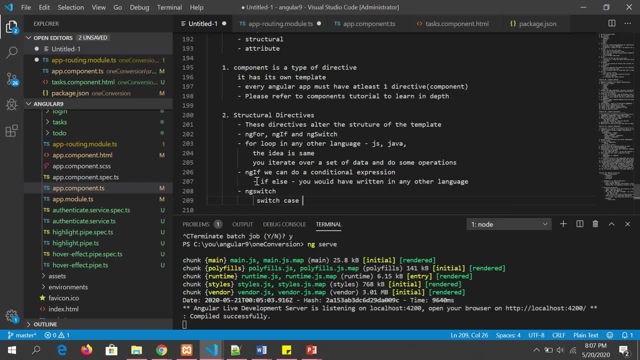 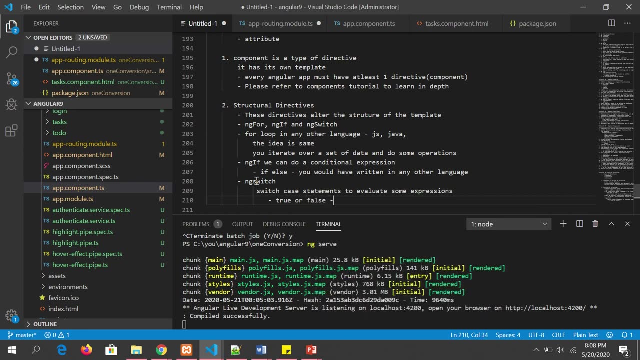 would have used in any programming languages. you would have used switch and case statements, uh- to evaluate, um, evaluate some, And then based on the condition output: uh, true or false. uh, we will see output. see corresponding output right. 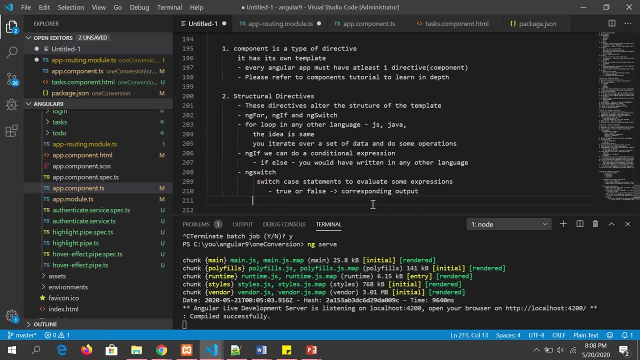 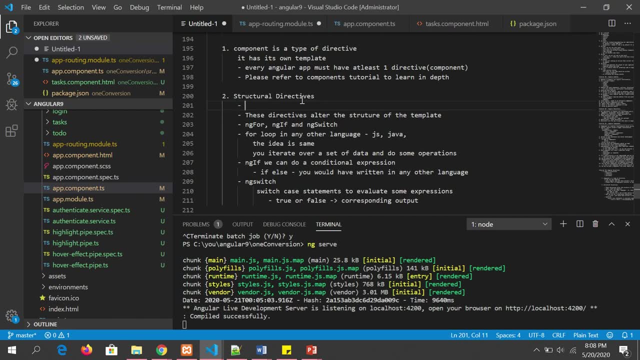 All right. So, that being said, how do you distinguish between the structural directives? So one of the most important things that you should know about structural directives is: they will always start with asterisk symbol. right, They will always start with asterisk symbol. 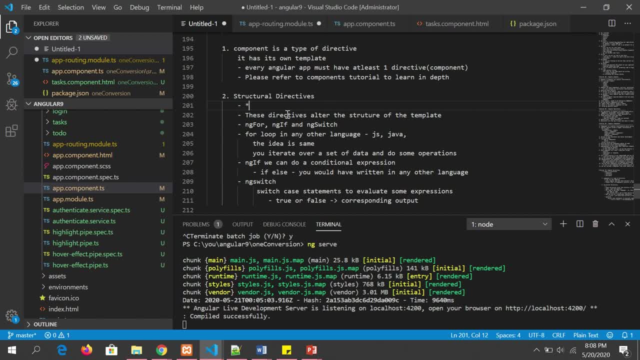 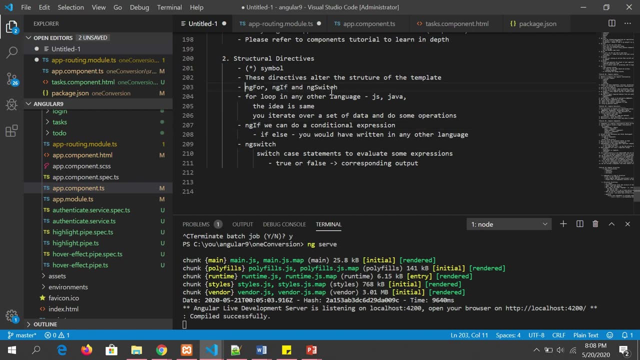 Now, if you see the code, it will always start with asterisk symbol. So this means they are structural directives or built-in directives, right? Uh, you can see that. So to use NG, for we'll say use NG, for we'll say NG for NG if NG switch. 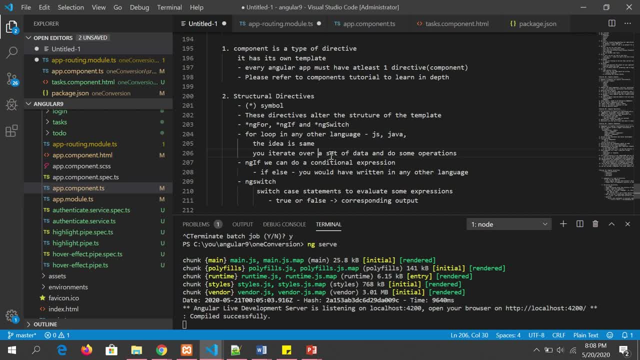 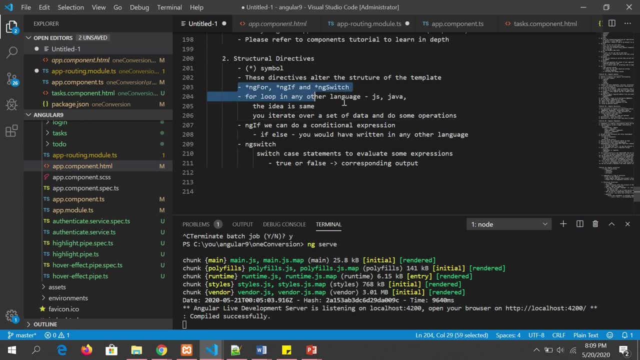 So this is how we write and declare the structural directives. I'll just show you a simple example And then, so don't worry, Um, we are going to cover all of this. They have a separate tutorial coming up for each. uh, in the next, that is tutorial number. 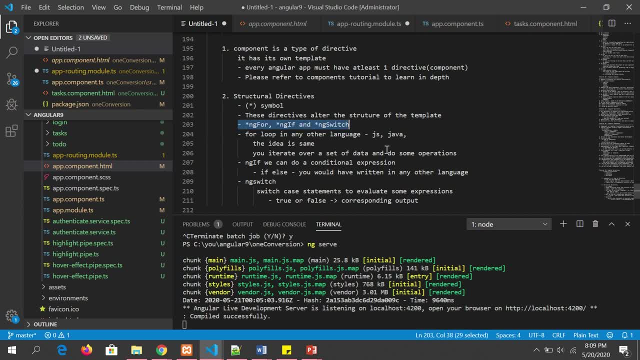 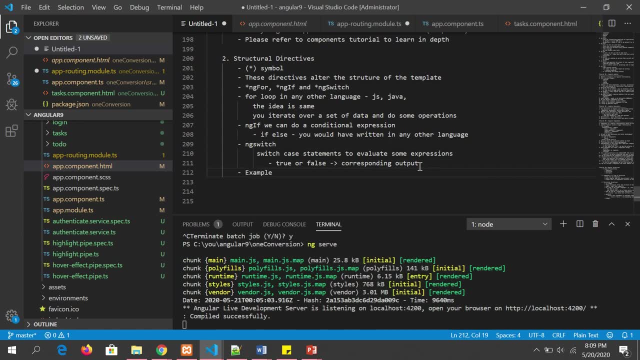 11,, 12, and 13 will cover NG for if and switch in detail, But just to give you a quick example: um, how do you, how do you use them? Let's do a quick example hands-on. 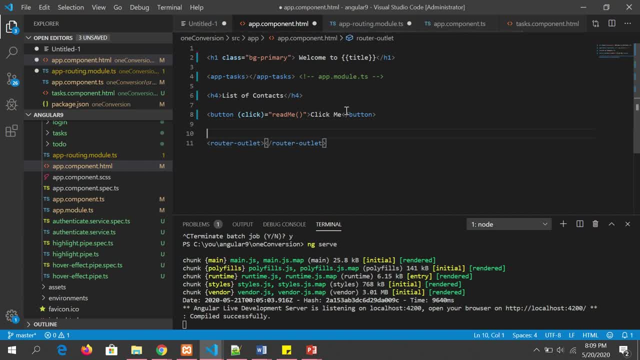 So let's open app component And here I'm going to just quickly throw in a- uh, let's throw in a DIV For now And NG if equal to expression, right? So here I'm saying: show message. If this is true, then show showing this message from: if true statement: right. 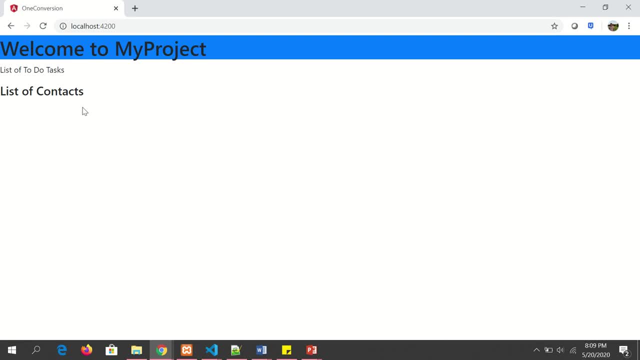 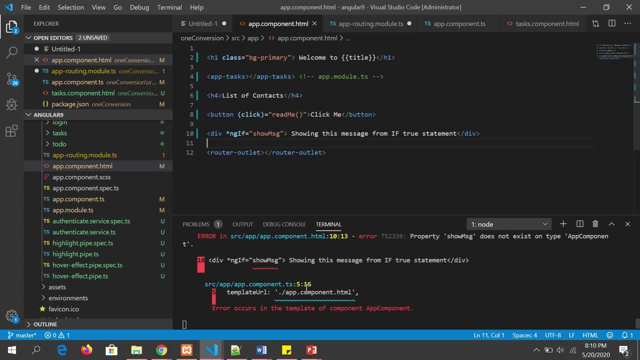 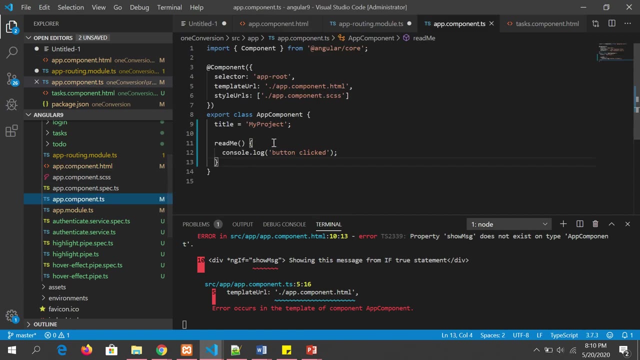 So if you see the output now, you would see that Okay, So we don't see. Okay, So what I'm so it says uh occurs in the template because show message is not defined. So let's go to our component and we'll put it here and I'll put it to false. 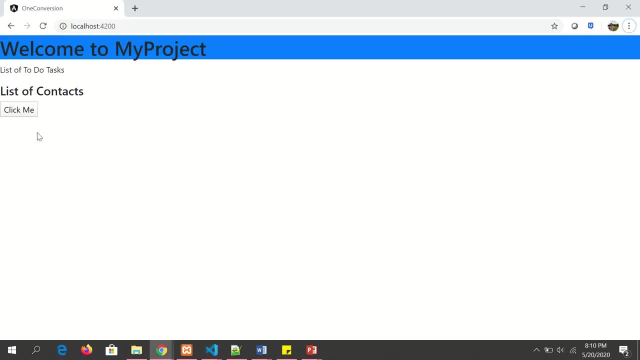 Okay, So now see it has successfully compiled. Now you open, you don't see it, The message I'm going to make it true. So showing this message from: if true statement: right, I made it true. And in the template: 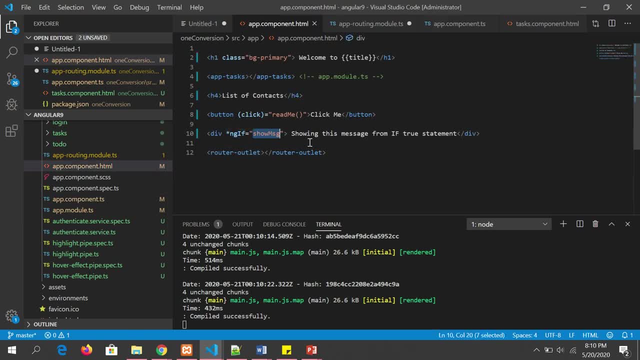 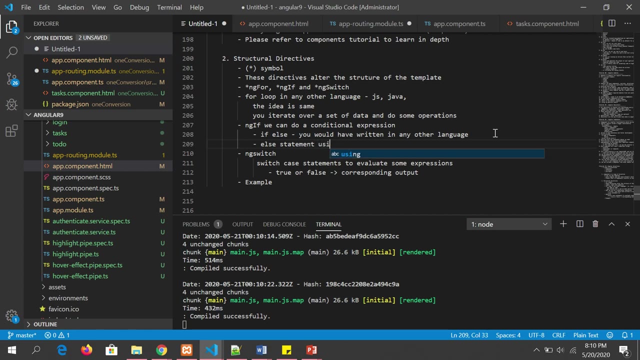 It is taking a structural directive called NG. If and if this message expression is true, then show this right. So there are a lot of combinations that you can do: Uh, for example, in the in the NG. if we can also define L statement, uh, using template. 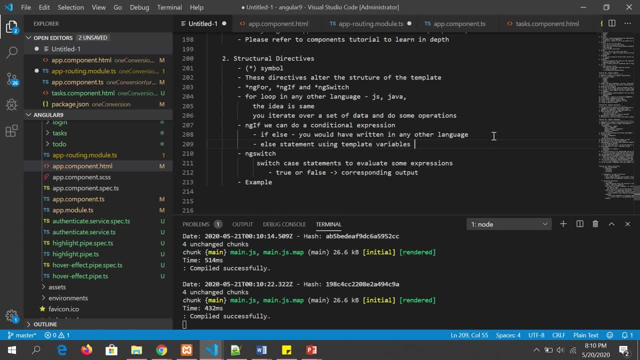 variables. uh, we'll learn about that in next tutorial. that's covered in tutorial 12.. That is the next tutorial, So stay tuned for that. So yeah, So coming back to so structural directive, There are three types: NG for NG. if NG switch, you can use them to change the structure. 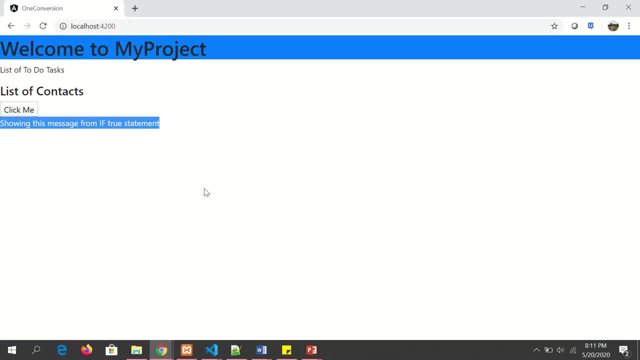 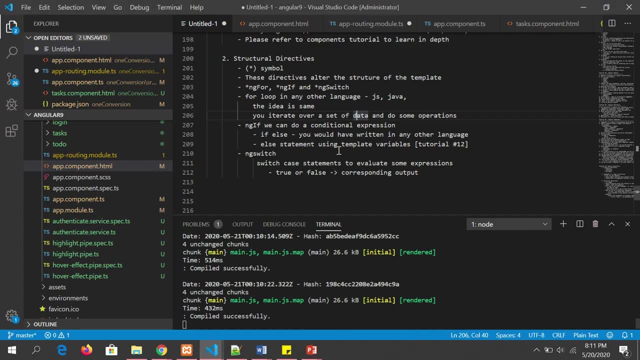 If you see here, based on this, it's changing the elements in the screen, You can show this message. You can hide this message based on a condition. right, So that is called as structural directives. Similarly, we will learn how to use NG for if and switch in detail. 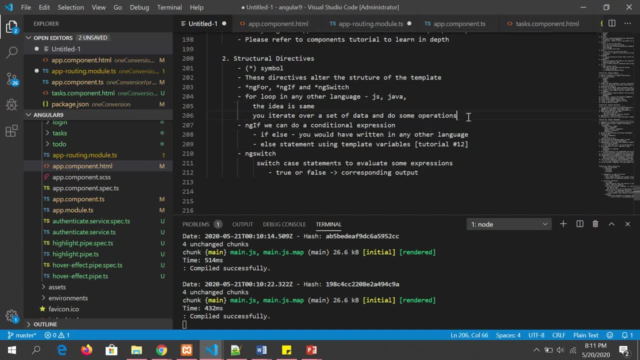 There are a lot of combinations that you can do with for loop Um, and you can use it in the next tutorial, And you can also do it with switch statements. We'll cover it in next uh tutorial, where I'm dedicating completely for that. 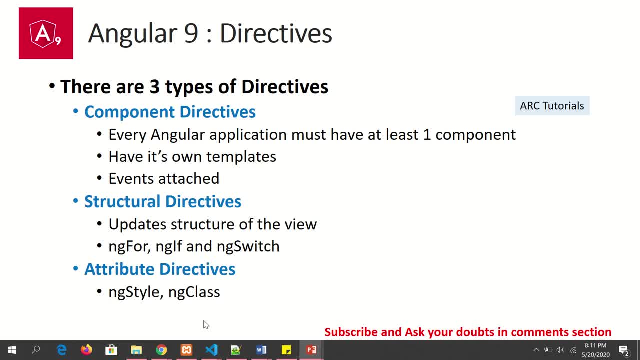 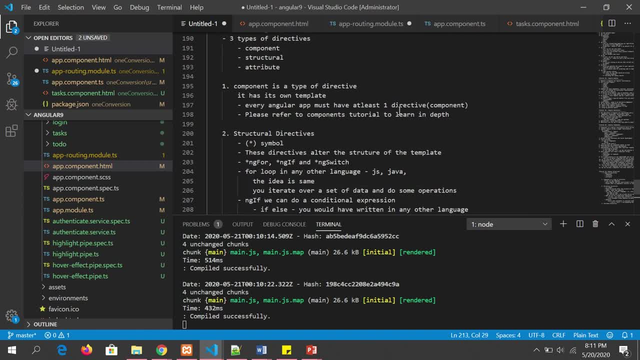 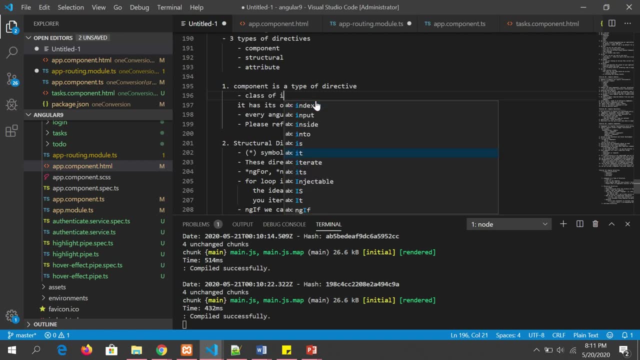 Let me also a little bit talk about attribute directives. Now, attribute directives are so we have seen. component directives are nothing, but they are class right. This is like a class of its own, component It's a class of its own, Whereas structural directives changes the structure right. 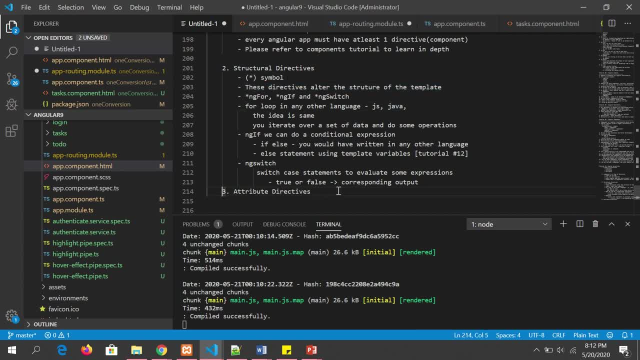 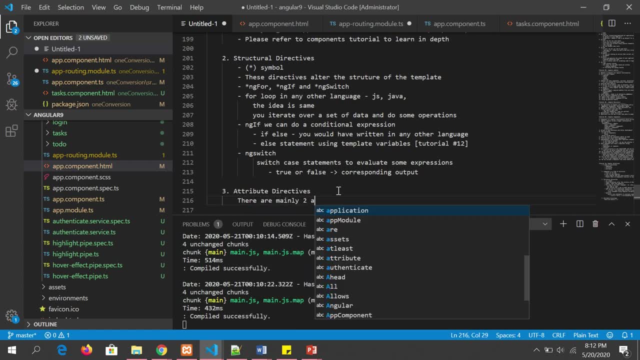 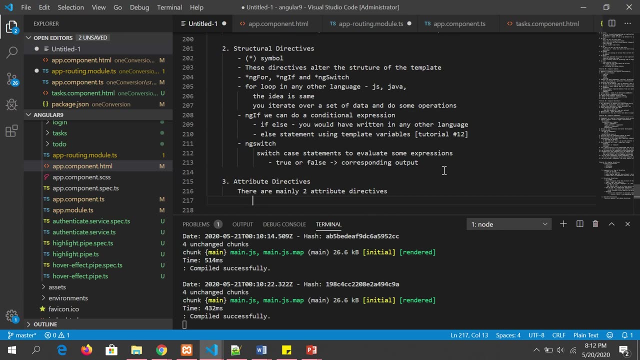 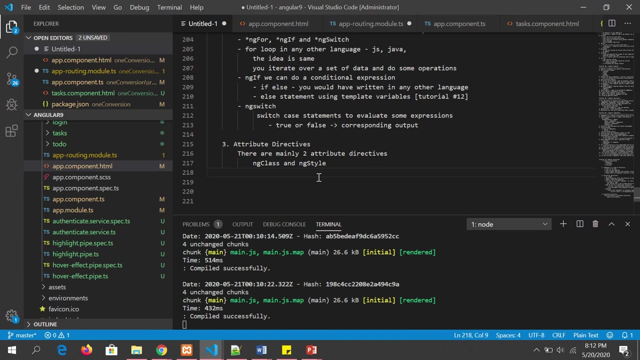 Or elements in the template attribute directives. We pass them along with the element. So there are two mainly. there are mainly two uh attribute directives that we use, attribute directives. One is NG class and the other is NG style. Again, we'll learn them in detail but for now let me show you an example of how to. 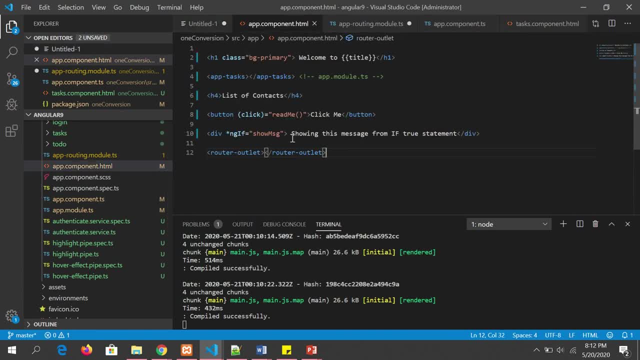 use them right. So again I'll go to my app component For this. Now let's say we want to add some uh style, right? So we can always say NG style equal to. so here I'm dynamically passing. 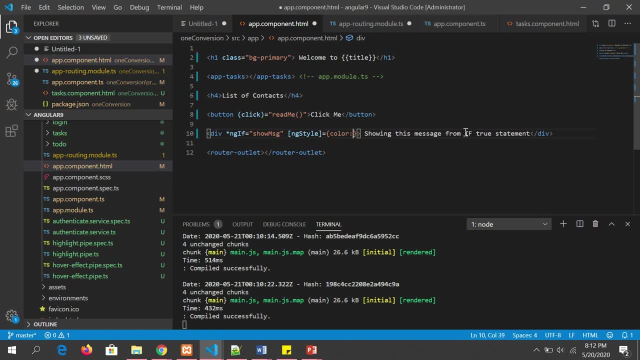 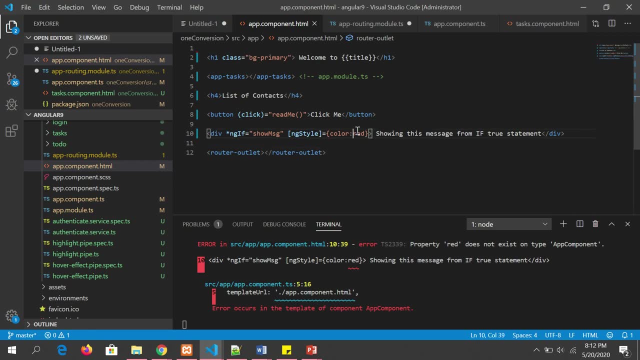 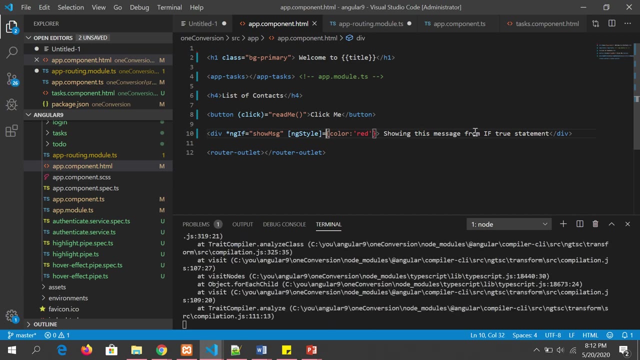 So here let me say NG style, let's say color: right, I can make it red, right? So there isn't seems to be an error, Okay, Okay, Sorry, Just give me a minute, Let me fix this query real quick. 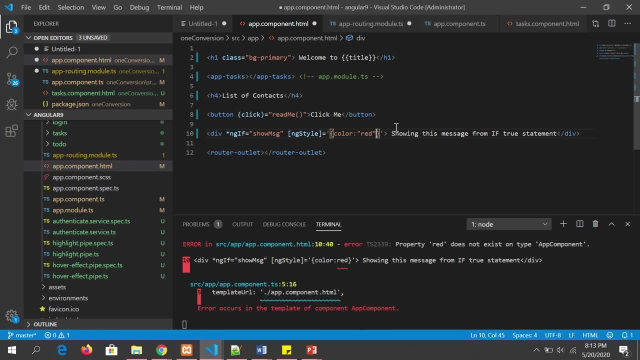 Okay, And then okay. So now I'm giving NG style and I've given color as red. So see, now this has become red color, right? So this is nothing but an attribute um directive, which is NG. Similarly, we can make it dynamic value also. 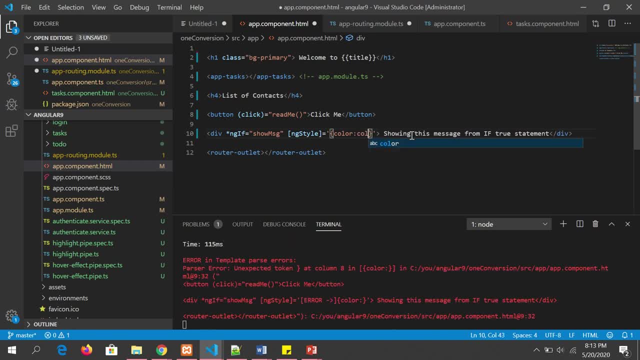 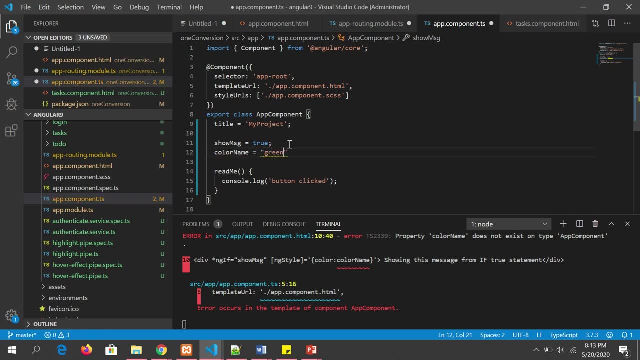 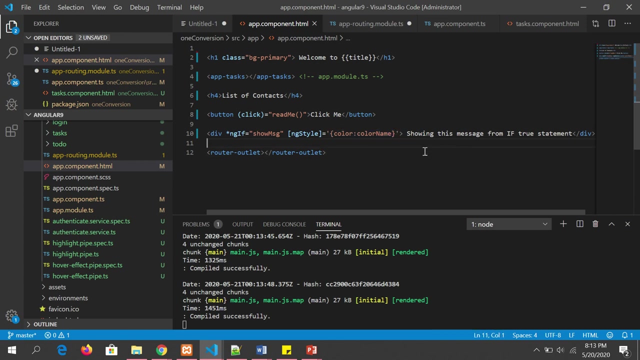 You don't want this here? No problem, Just say color name and let's grab it here. Put it here: say green, right. So now I've given color name as a variable, which is green. Now I'm using that here in the expression which is inside this uh bracket. 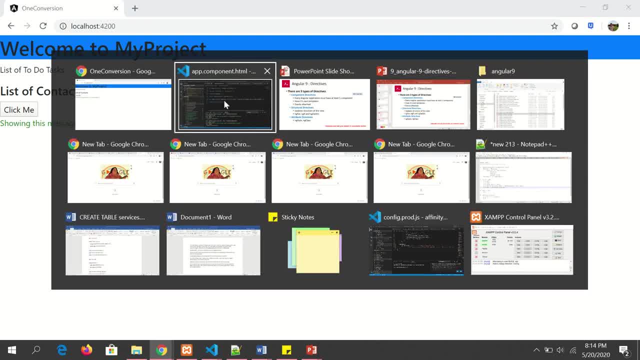 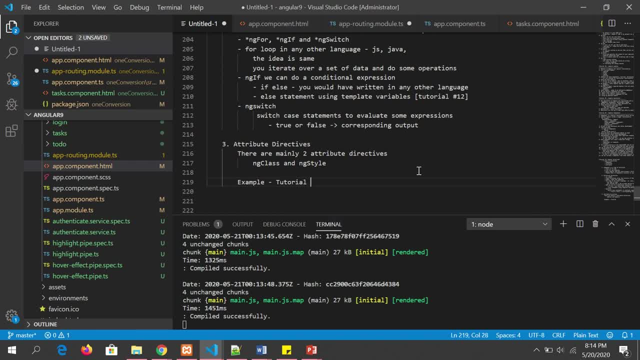 Now you see, the message is green, right, So this is how, uh uh, structural directives work. I'm sorry, Attribute directives work, but again, these are covered in tutorial number 14. So that's going to come up. 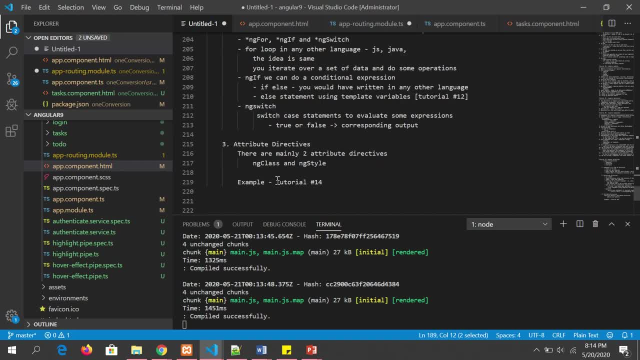 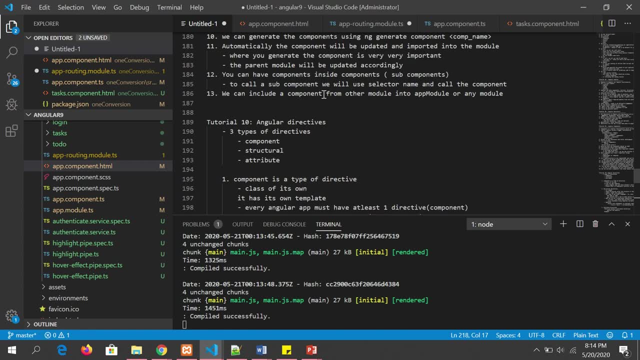 We are in tutorial number 10.. So this is to. we'll cover all of this in detail. Um, so don't worry if you don't understand. just this was only about the concepts. Um, so this was only about overview and concepts- understanding, right. 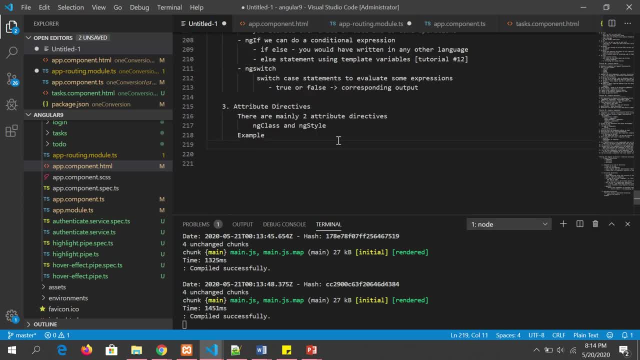 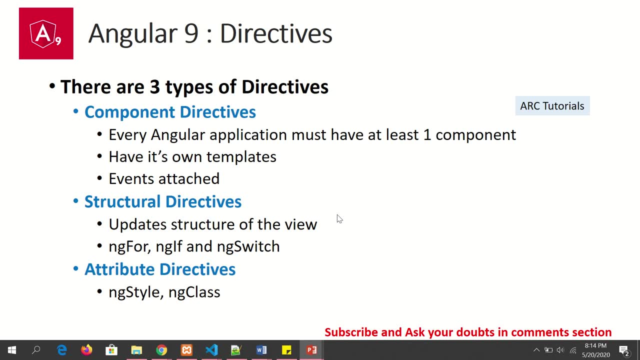 Okay, Uh, we'll do all of the practical hands-on in the next uh tutorial when I'm covering NG4, starting with NG4.. All right, So that brings us to uh the overview of directives. So there are typical uh three types of directives: component directives, structural. 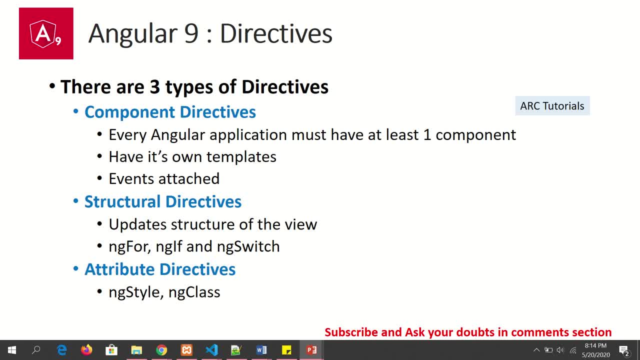 directives and attribute directives. Component directives We have seen in component tutorial. every application must have at least one component. You can generate any number of components that we want. Structural. Structural directives are something which will update the structure of the view. 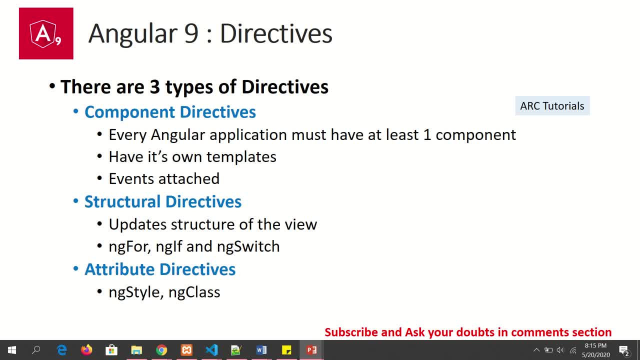 There are three types of structural directives: NG4, NGif and NGswitch. We also have attribute directives, NGstyle and NGclass right. So these are the attributes which are used to basically change the styling property. To identify structural directives, we'll use asterisk symbol right. 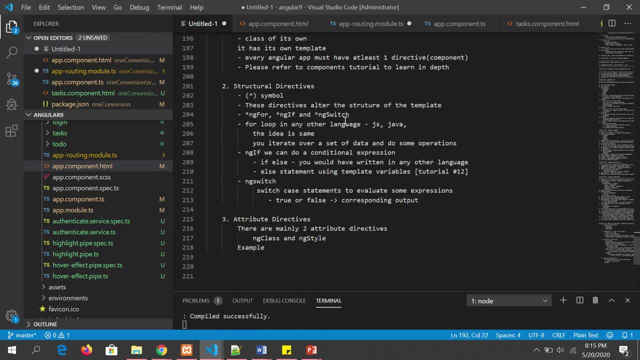 So that's what we made in the notes here. Just go through this. Let me know if you want this. uh, change the color using NGstyle. That's what we did in example. now, All right, So this is the notes that we had. 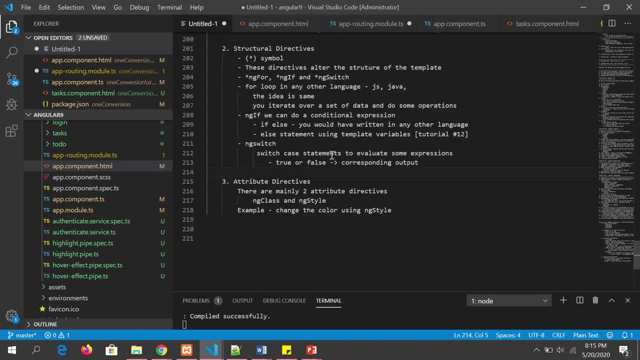 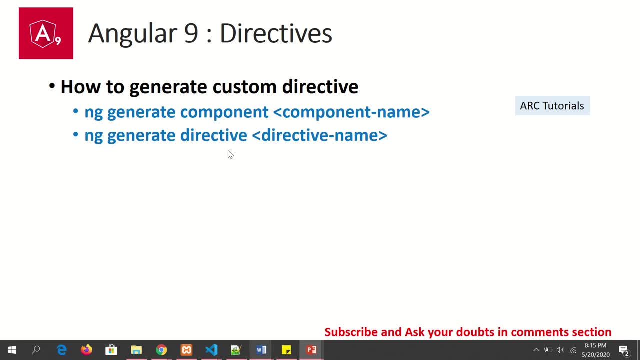 Go through this notes. go through the tutorial: um in the next, uh upcoming tutorial: Um. so yeah, this is uh. I forgot to add one more thing, So this is a bonus component, I will tell you. but again, this is for advanced thing. 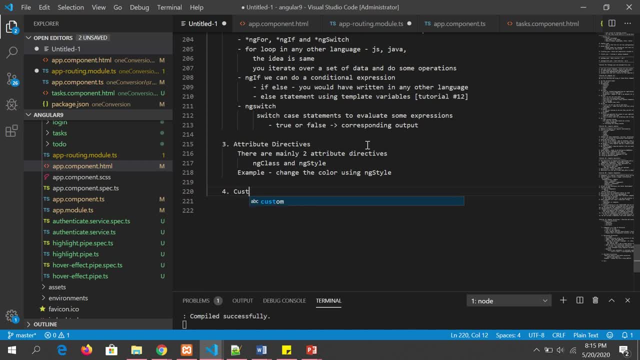 Don't take it too hard yet, We will cover it. Uh, then we can also generate custom directives. We can generate custom directives. So this is like adding more power and extending our ex application using custom directives, right? Um, we can. we can generate using NG. generate command, uh, directive and followed by directive. 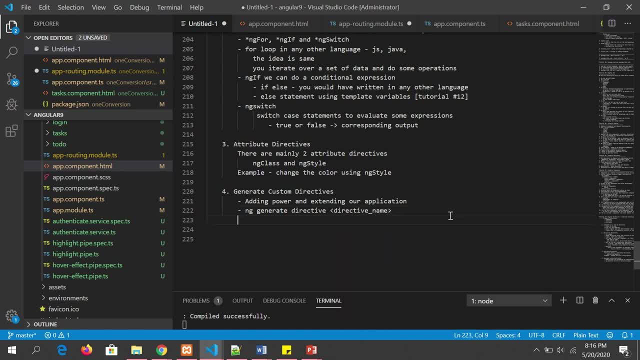 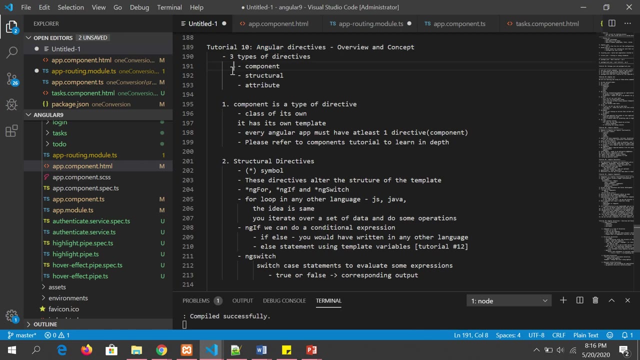 name. Uh, like I said, do not go into the details now on this because this requires a topic and a separate tutorial. on its own, It's little um advanced concept for now. I want you to start with tutorial angular directives and understand these three first. 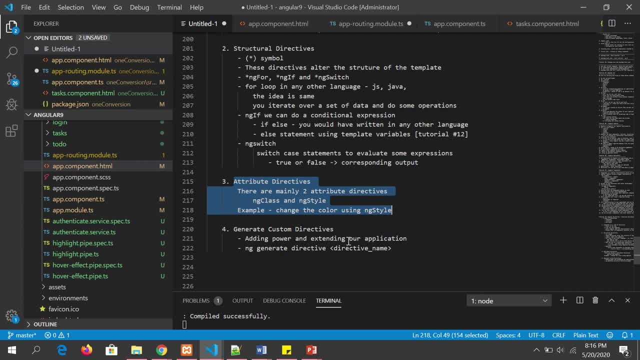 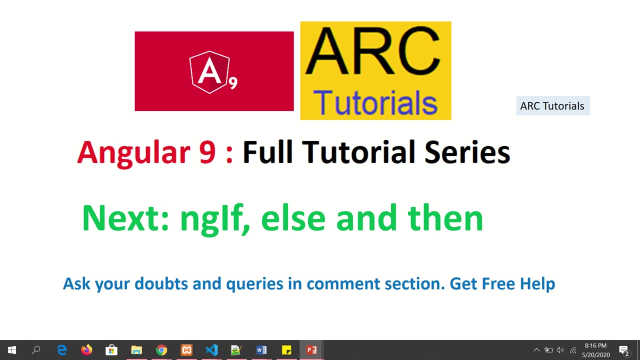 that is, component directive, structural and attribute custom directive. We will do it later in the tutorials where we cover full-fledged, uh, dedicated episodes for it. All right. So that being said, uh, in the next tutorial we'll cover about NG, if else else and then.